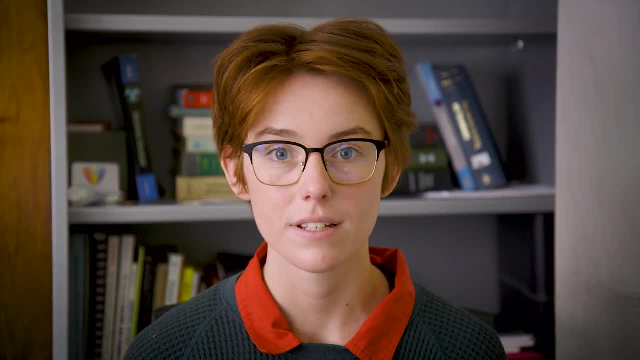 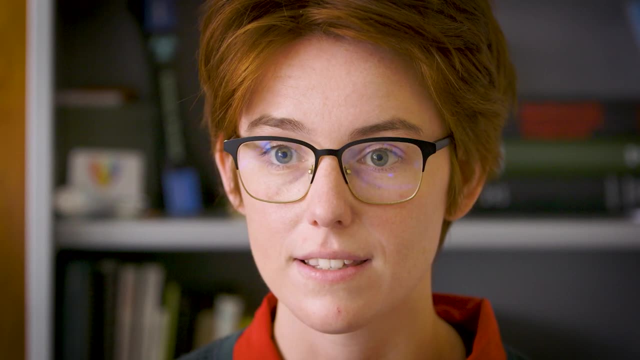 inside of a nuclear reactor. We track neutrons as they bounce around computationally inside of a simulation. We watch them scatter. We watch them produce fissions. A particularly interesting type of neutron, the one that pertains to my particular work, is slow-moving. 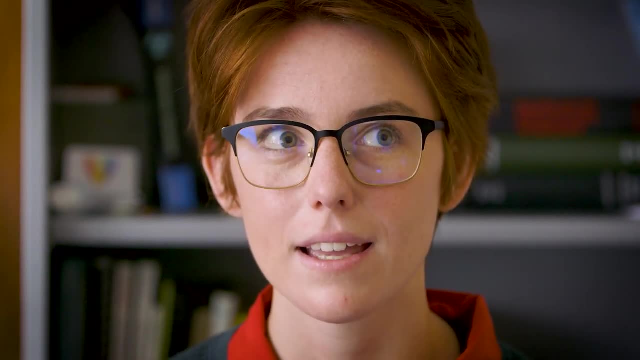 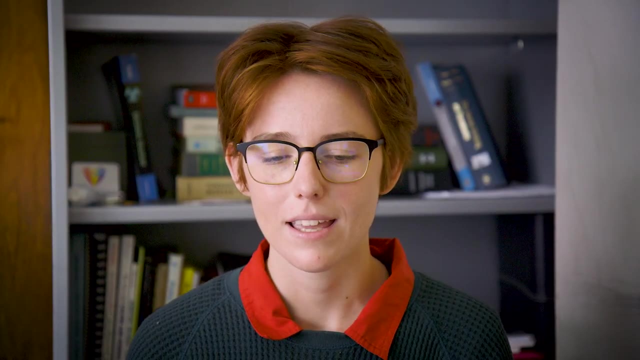 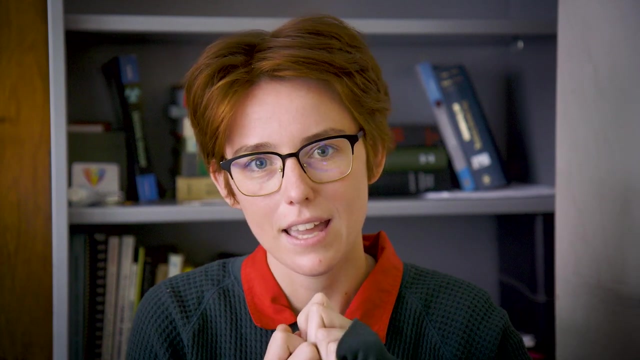 neutrons. Slow-moving neutrons abide by a little bit more special physics than fast-moving neutrons. If a fast-moving neutron hits an atom, it can just basically blast that atom out of its molecular bonds. It's going so fast that it can hit an atom and just kind of knock it out of the park. 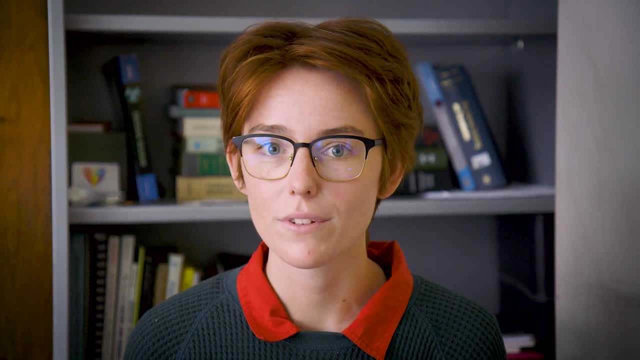 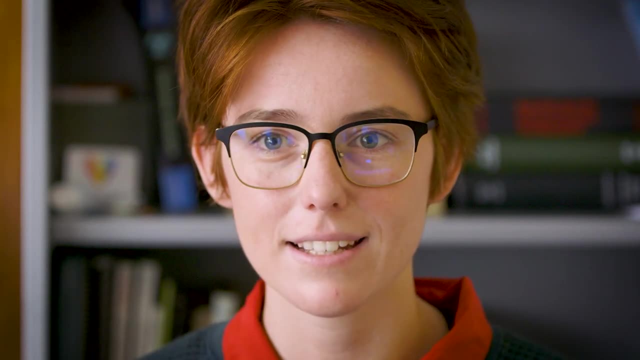 ignoring molecular bonds that might be holding it in place. Slow-moving neutrons are way more interesting. They will tap this atom as it's being held by its molecular bonds or inside of a lattice, And instead of just knocking this atom out of its place, it'll 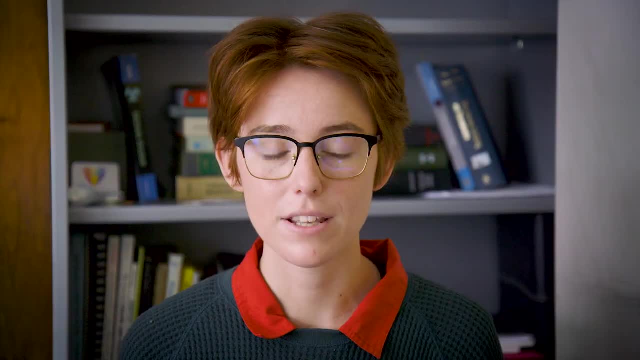 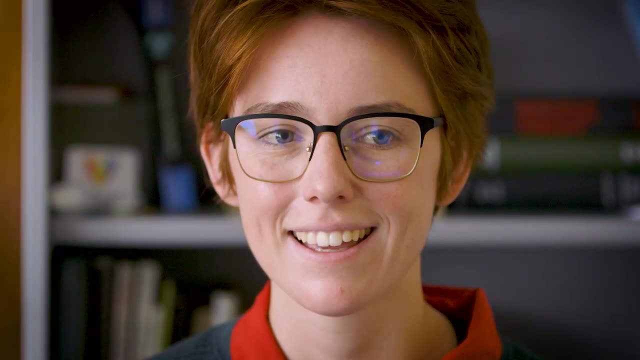 induce vibrations. It will jiggle this atom around, And so my job is to try and account for those little vibrations that will be induced by a slow neutron just kind of tapping it. So I'm going to show you how that works. I'm going to show you how that works. I'm going 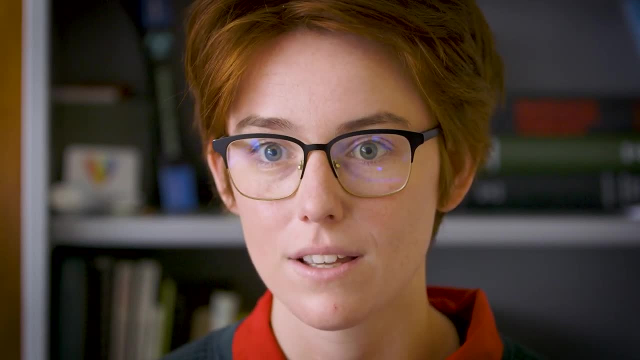 to show you how that works. It opens up a really interesting type of physics, one that I care deeply about. 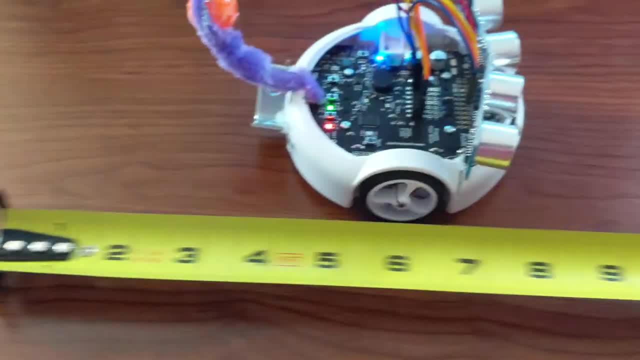 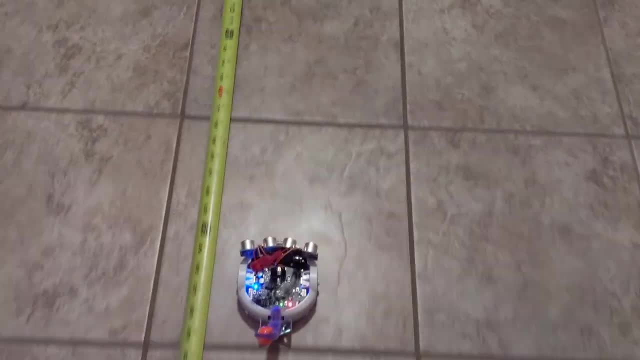 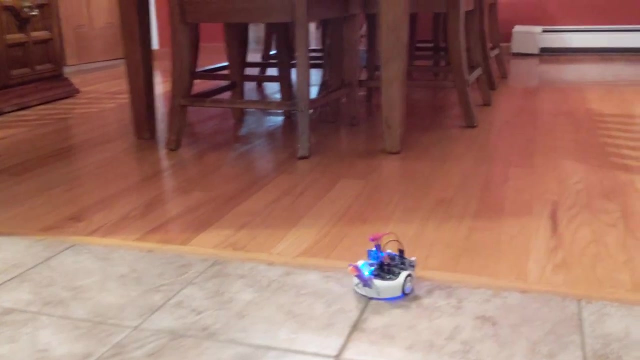 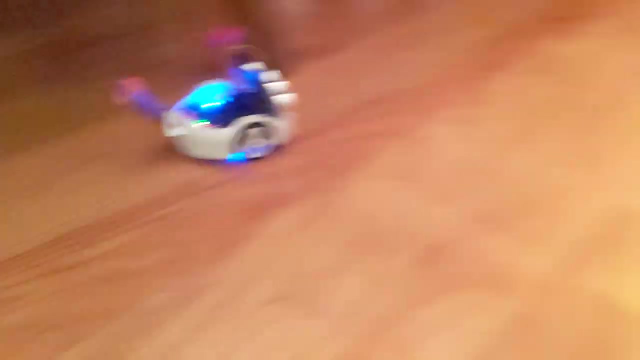 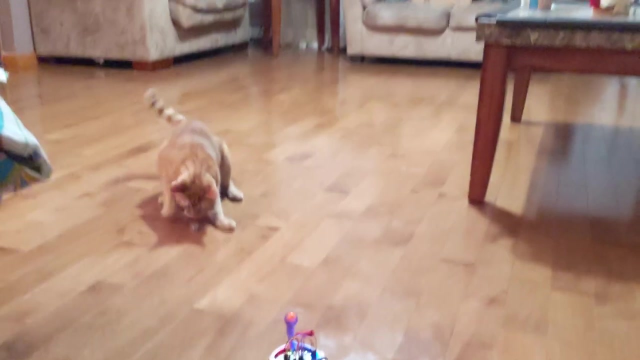 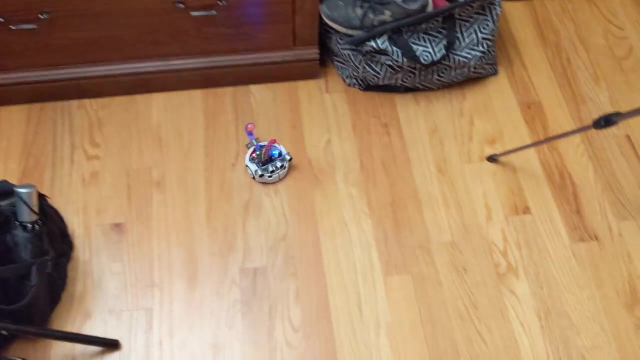 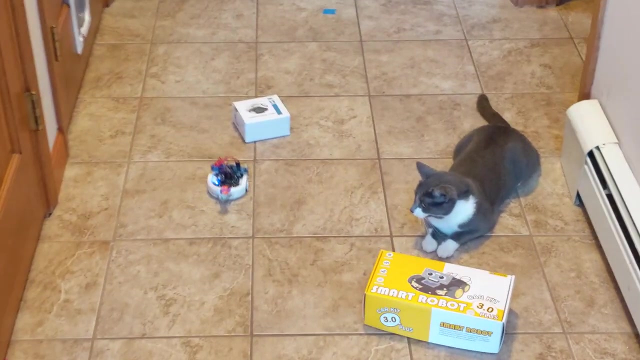 Please subscribe to the channel and press the bell icon to receive notifications when I upload a new video. Thank you for watching. Please subscribe to the channel and press the bell icon to receive notifications when I upload a new video. Thank you for watching. Please subscribe to the channel and press the bell icon to receive notifications when I upload a new video.